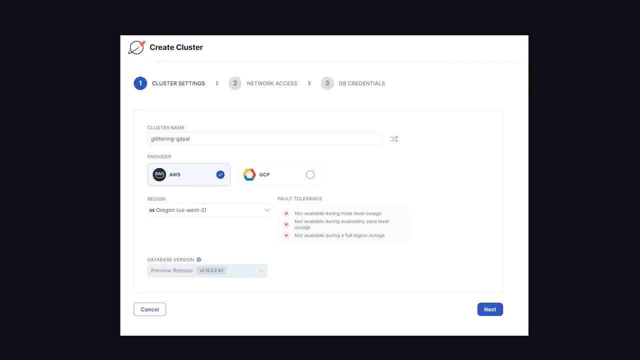 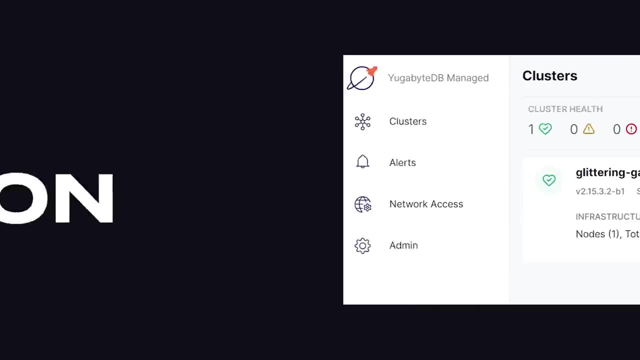 which is not easy to do in a cloud-native environment. You can actually use a multi-cloud strategy to host your database on multiple clouds at the same time eliminating the dreaded vendor lock-in issue. But there's another option for scaling Postgres, called Neon. 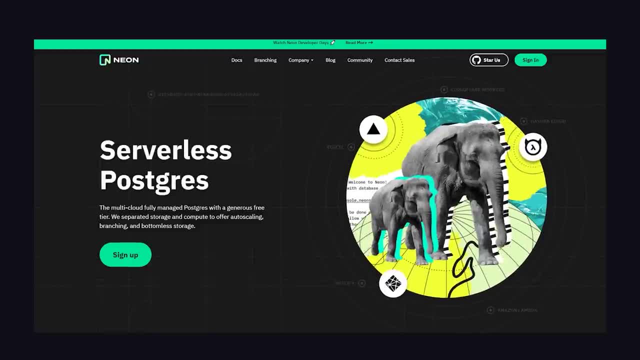 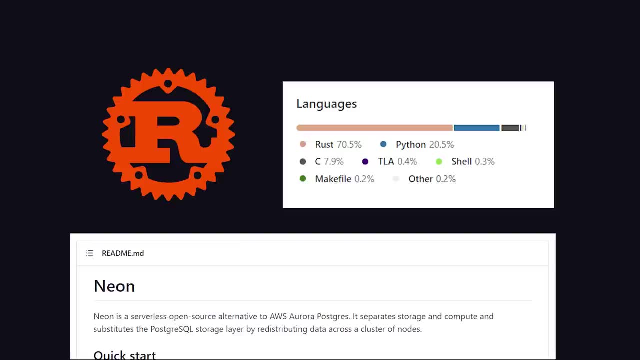 It's currently in technical preview, but looks extremely promising. It's serverless and can scale down to zero, and has a highly polished admin dashboard to go along with it. And, most importantly, it's written in Rust, which is the only thing that matters if you want to look cool in front of your friends. 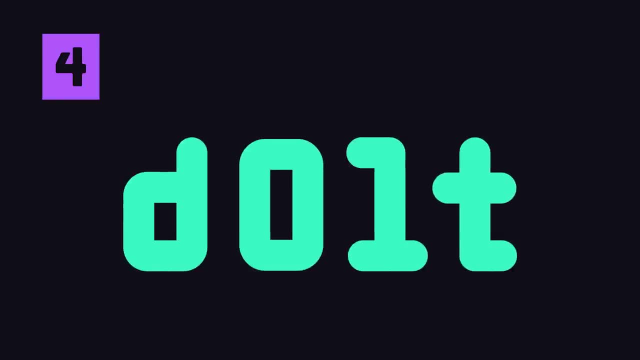 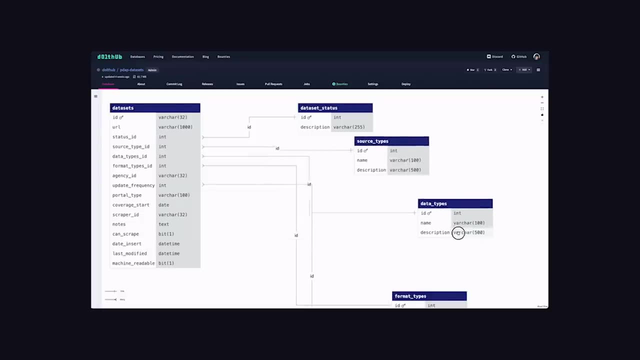 It also supports branching, which I think was inspired by another database called DOLT. This database would be like if MySQL and Git had a baby. Most importantly, it allows you to create branches from the main database where you can experiment with new data without breaking things. 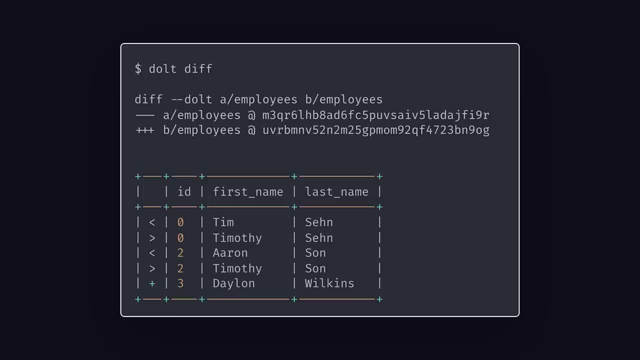 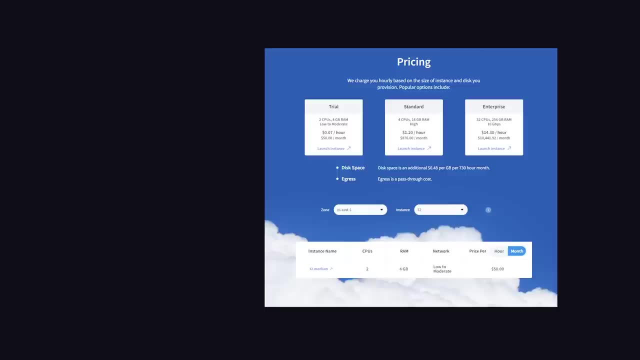 It makes it easy to analyze the diff between changes, and when everything looks good, the changes can be merged back into the main branch, And it's done with the same conventions found in Git that virtually every developer is familiar with. DOLT has a hosted option, but it is quite expensive. They've raised $21 million and because I'm extremely entitled, I demand they burn more of this money to give us a free tier. I just paid $8 for a dozen eggs and can't afford to put another $50 on my mom's credit card. 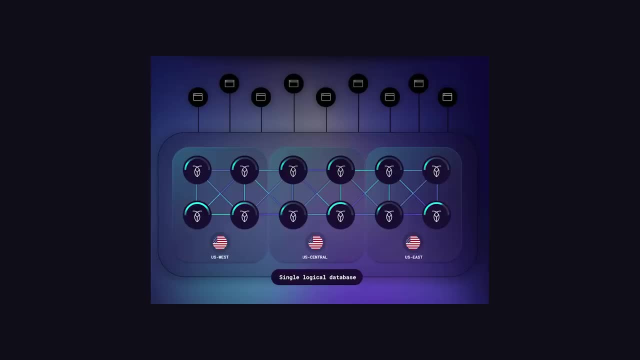 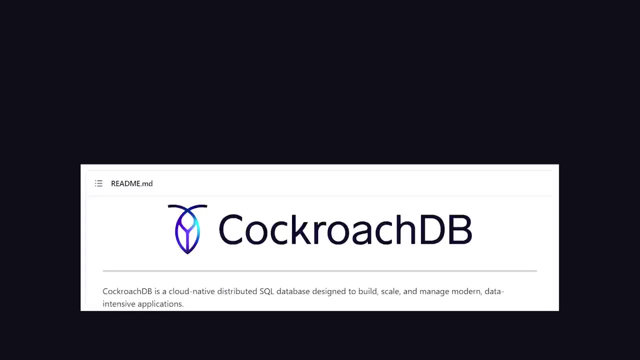 Now another SQL flavor I want to talk about is CockroachDB. It's been around for quite a while and was developed by ex-Google employees and is often referred to as NewSQL. It's compatible with Postgres, but was built from the ground up with Go. 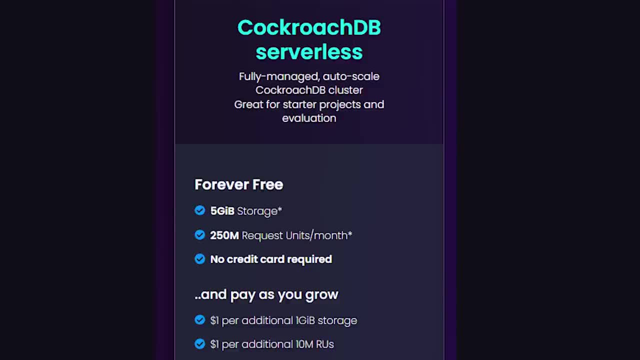 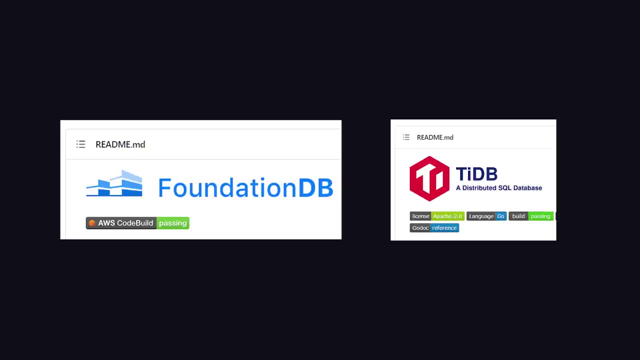 to scale horizontally in the cloud. It has a nice free tier, pretty similar to PlanetScale, then becomes pay-as-you-go pricing after that It's yet another great option. but you might also want to consider FoundationDB or TitaniumDB as well. 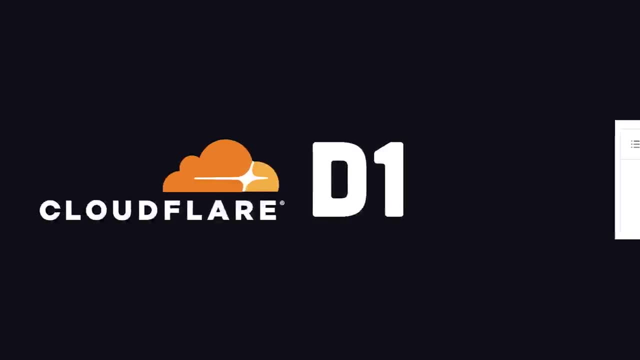 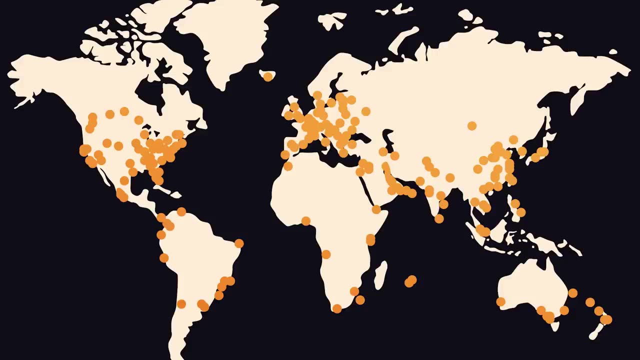 which are also in this NewSQL class, But in some cases you might prefer a lightweight alternative like Cloudflare D1.. This is a brand new product that's still in beta and basically it's a SQLite database that runs on the edge. 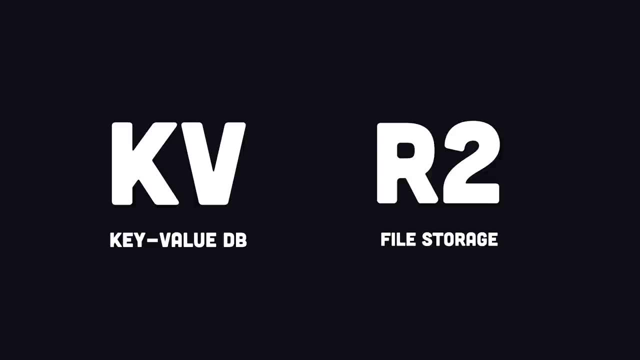 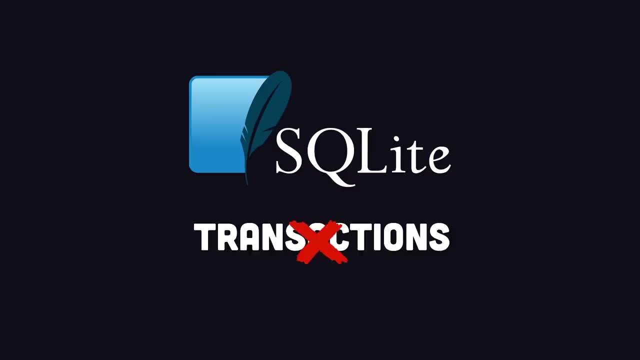 Cloudflare already has its own key value store for workers, as well as R2 for object storage, but D1 allows you to create data on the edge, so you don't have to worry too much about it. One trade-off, though, is that native transactions will not work. 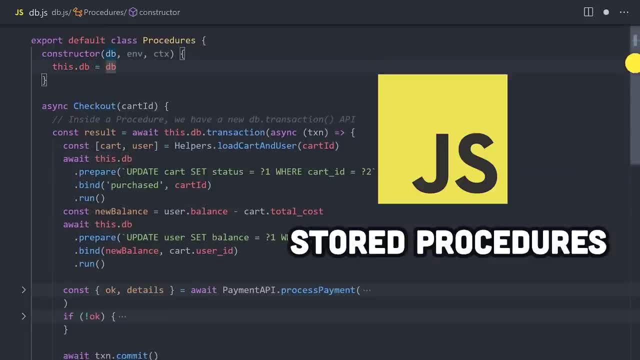 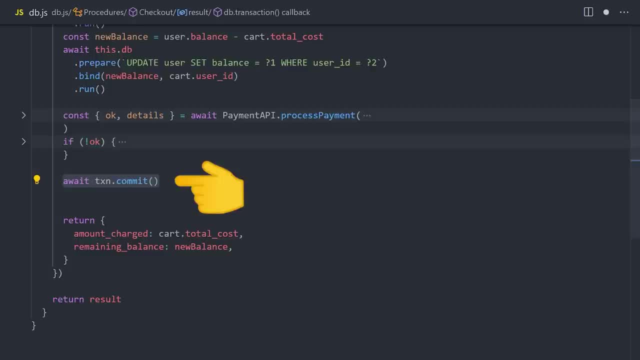 However, they're taking a very cool approach to overcome that limitation by allowing developers to write stored procedures with JavaScript, which are just snippets of code that run directly in your database, which can be used to create transactions or other reusable queries. This approach has a ton of potential, because, historically, stored procedures are a pain to work with. 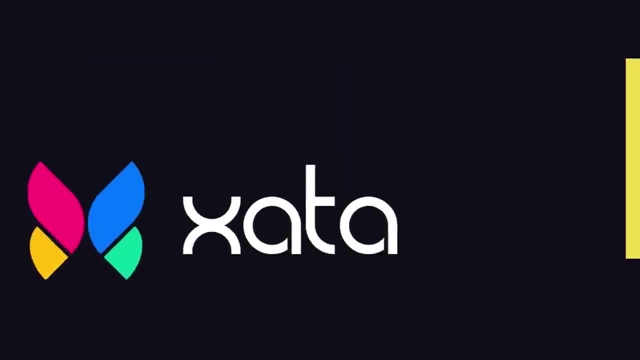 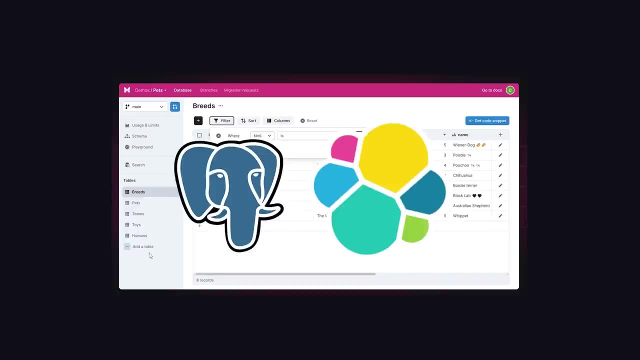 But if it's in JavaScript, even I could do it- Pretty cool, but it's not production ready yet. If you want something that's ready to go today, check out Zeta, yet another serverless relational database that's based on Postgres and Elasticsearch under the hood. 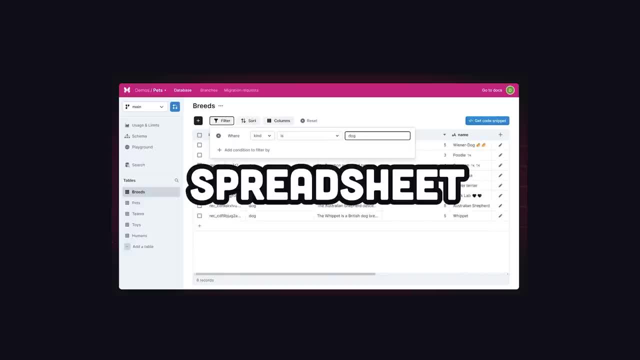 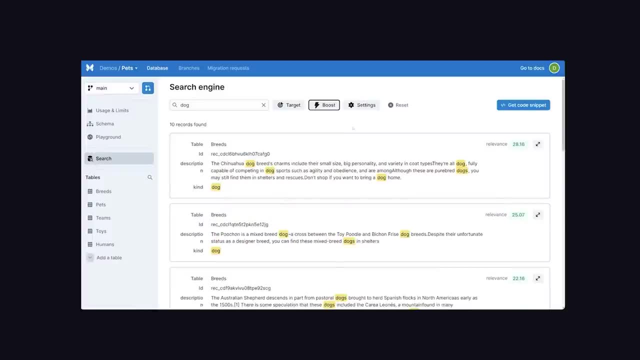 What makes it special is that it treats your data like a spreadsheet. It feels kind of like a developer-friendly alternative to Airtable or Notion, And what's really awesome is that it has full-text search built in without needing to duplicate your data in some other service like Algolia. 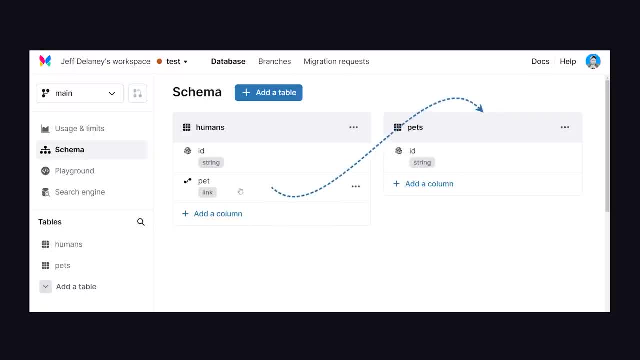 It has SDKs for TypeScript and Python and has a schema editor that makes it very easy to create and visualize relationships between tables, And it can also do branching, like we looked at in DoltDB. For pricing, it has a solid free tier. 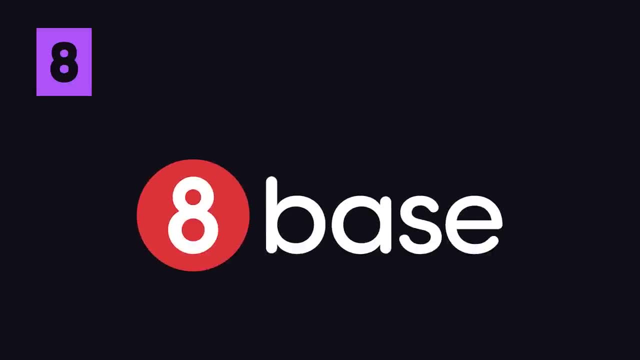 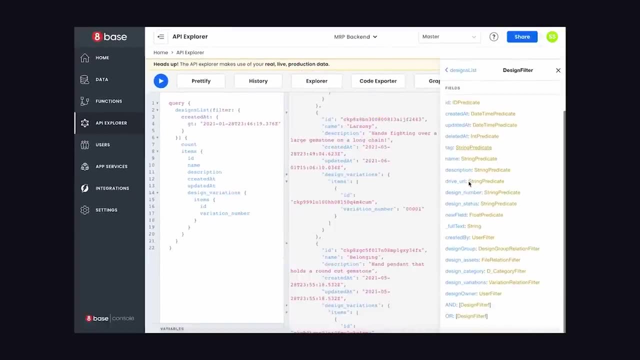 Then it scales up in a linear way based on usage. But another tool that takes things one step further is 8Base. It's also a relational database that provides a GraphQL API for your data out of the box, making it similar to tools like Hasura. 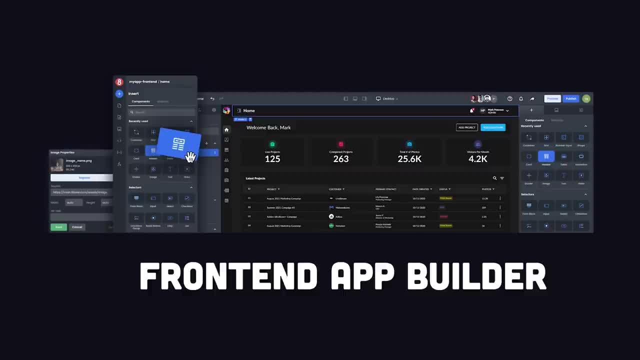 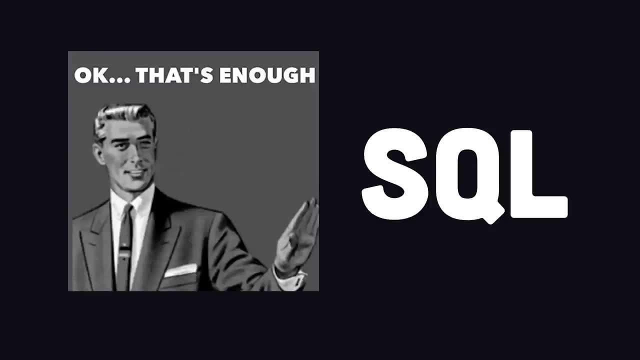 What makes it unique, though, is that it also comes with a low-code tool for quickly building front-end applications that connect to your back-end. It's like a back-end-as-a-service that can also build your front-end, But that's enough. talk about relational databases. 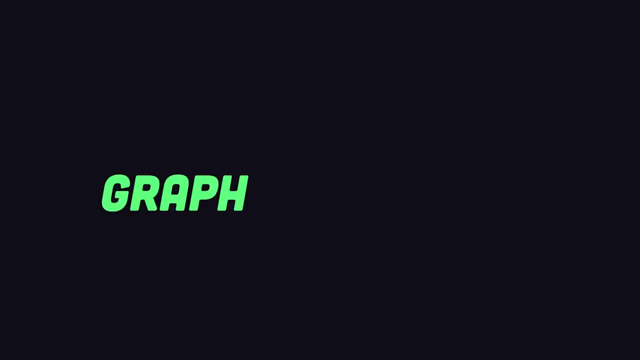 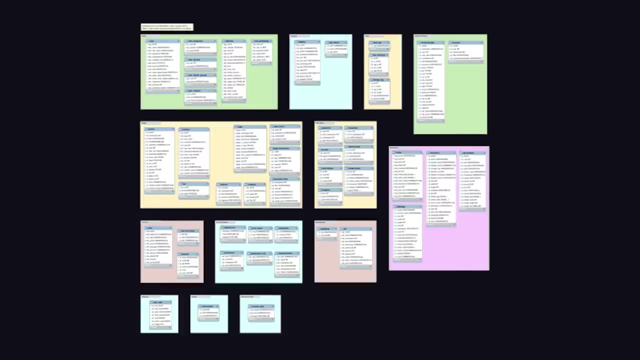 Now we enter the PostSQL era with EdgeDB. It's a graph relational database that's powered by Postgres under the hood. When it comes to relationships, humans don't naturally think of columns and rows, but rather objects connected to each other like a graph. 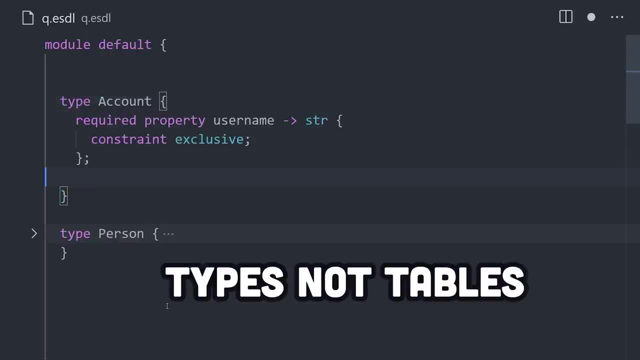 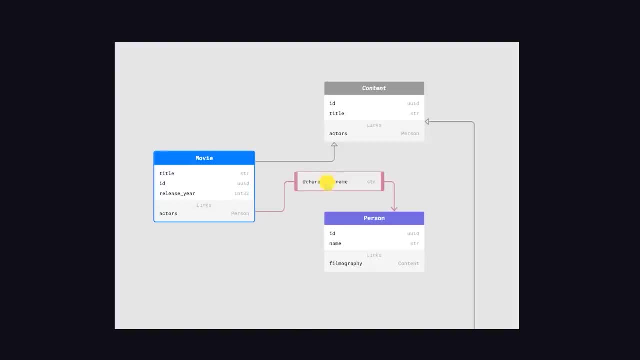 Instead of defining tables, like you would in SQL, you define types, like you would in most programming languages. These types link to other types, which is awesome because it eliminates the need for joins and simplifies the way you make queries. Overall, it almost feels like an ORM for Postgres. 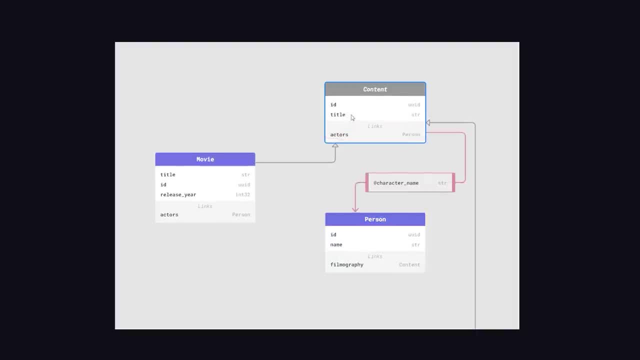 that allows you to think about relationships in a far more human-friendly way. Currently it's open-source and can be self-hosted, but there's a waitlist for their cloud service. Now another relational graph like EdgeDB, which is based on PostgreSQL, is also based on PostgreSQL. 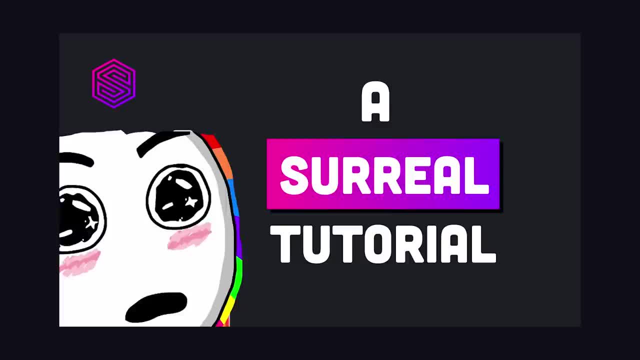 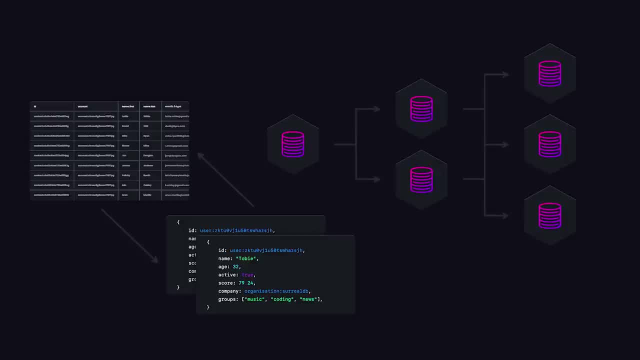 Another relational graph like Database is SurrealDB. It's written in Rust and I have a full tutorial on my second channel Beyond Fireship. It's designed to support ACID transactions while scaling horizontally, but what I really like about it is how easy and flexible it makes data modeling. 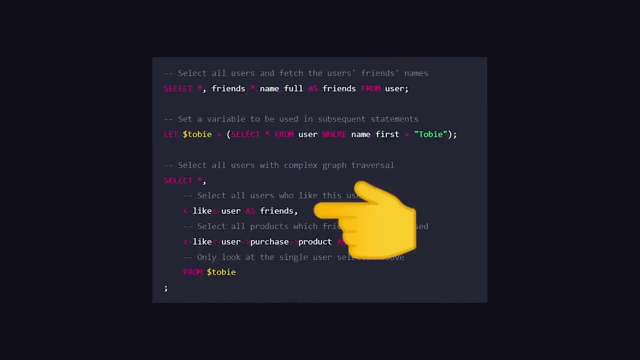 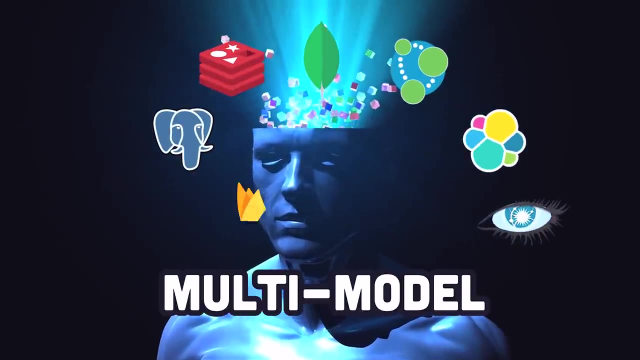 For the most part it feels like SQL, but also uses arrows to connect nodes and edges, like you would in Cypher with a graph database like Neo4j. It takes the best elements of relational document and graph databases and combines them into one easy-to-use API. 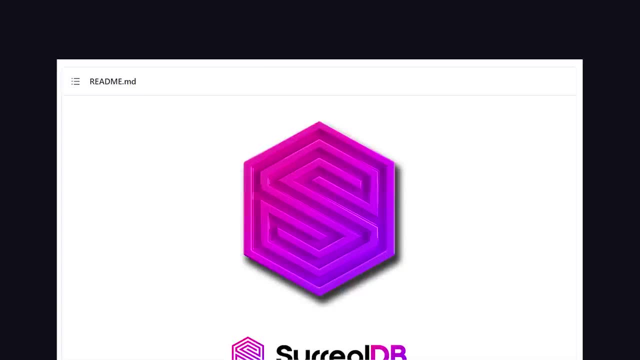 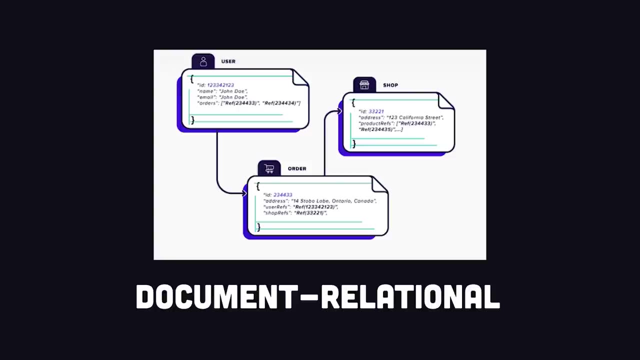 Currently it can only be self-hosted, but they do have a cloud service coming soon. The multi-model idea is nothing new, though. Another database pushing the limits is Fauna. It was created by ex-Twitter engineers who set out to build the perfect database. 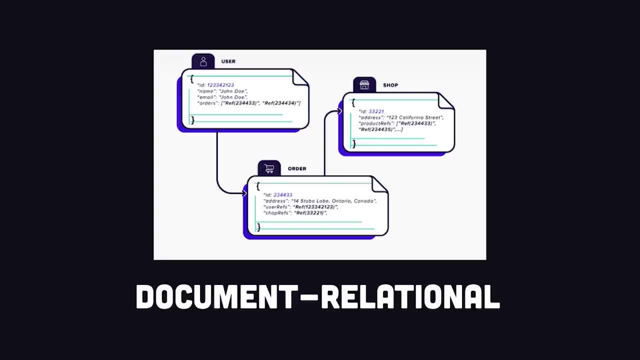 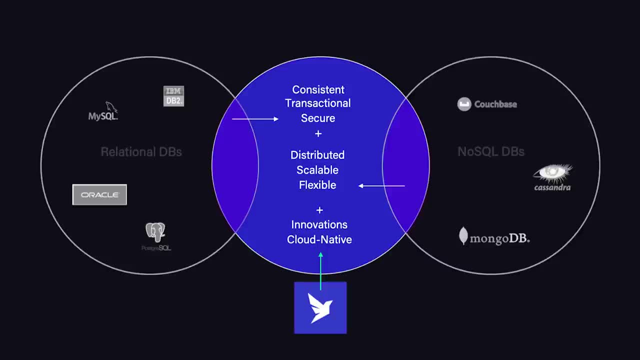 It's extremely easy to use like a document database, similar to MongoDB, but unlike a document database, it supports features like native joins, which is the number one missing feature in document databases, And that means Fauna is more well-suited for complex relational data like social graphs. 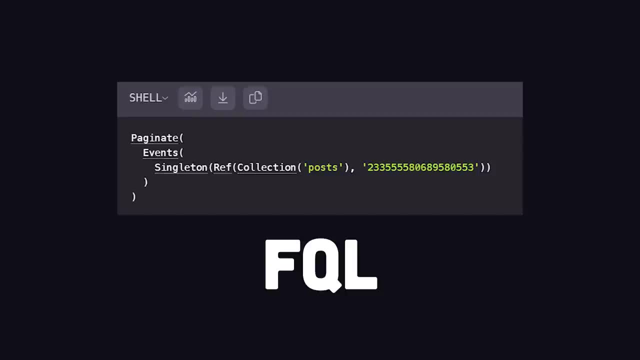 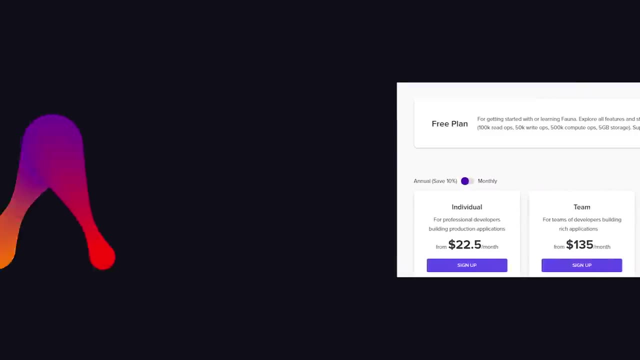 To interact with it. it has its own custom query language called FQL, but also comes with a GraphQL API. It is a closed-source product so you can't self-host it, but its fully-managed service has a nice free tier. 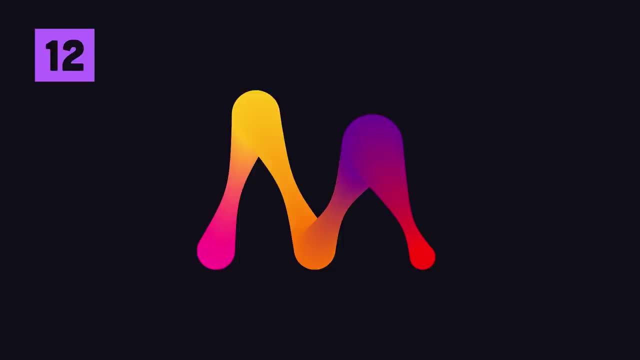 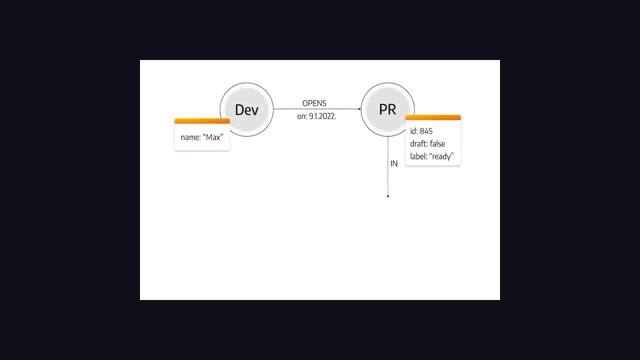 Another new database you've likely never heard of is Memgraph. It's a drop-in replacement for Neo4j, which is the gold standard for graph databases, but Memgraph is focused on building real-time data pipelines. Like Neo4j, it can be queried with Cypher. 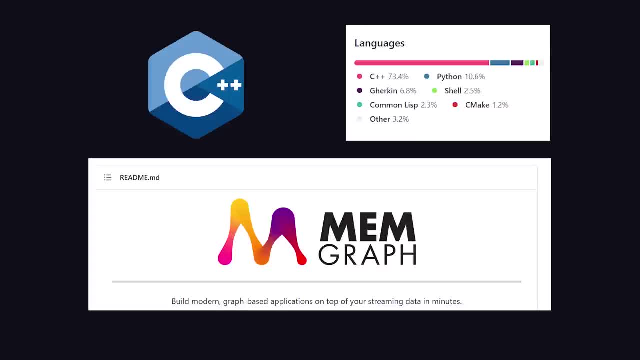 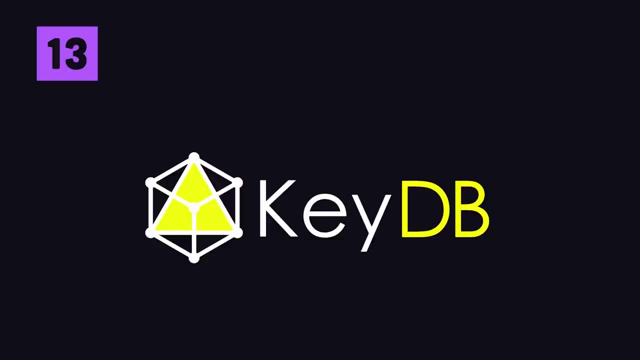 but it's written in C++ with a memory-first architecture that claims to achieve better performance. Overall, it looks like it would be a great choice for building something like a real-time analytics platform. Next up, we'll look at KeyDB, which is a faster alternative to the extremely fast Redis. It was recently acquired by Snap, a company that needs to fetch data as fast as humanly possible. It can handle over 1 million operations per second on a single node, which sounds like a lot to me, but it's not something you would use as your primary database. 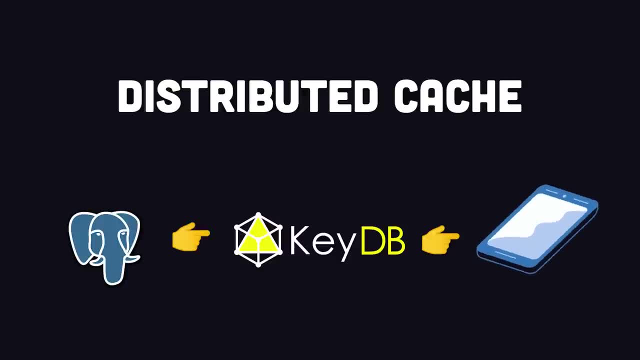 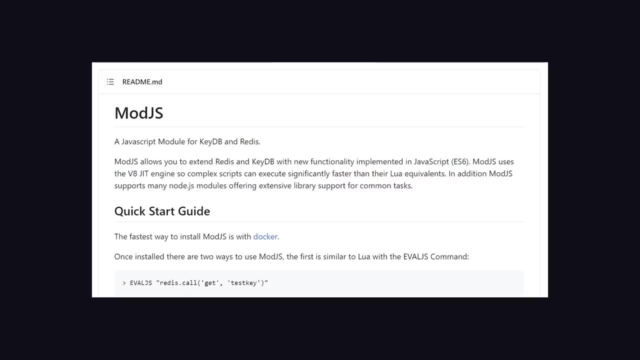 Rather, it's mostly used as an in-memory cache to duplicate high-priority data from another database, making it load faster for the end user. It also has a library called Modjs allowing you to extend the database with your own custom commands and functionality with JavaScript. 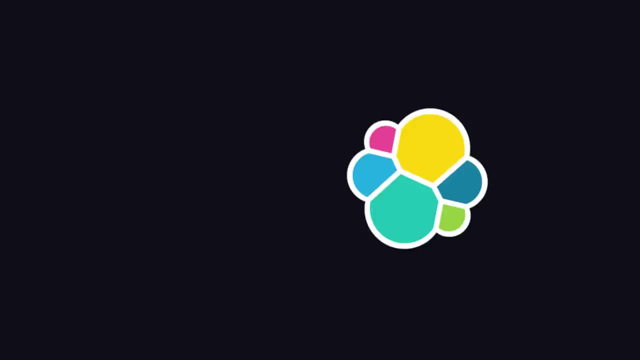 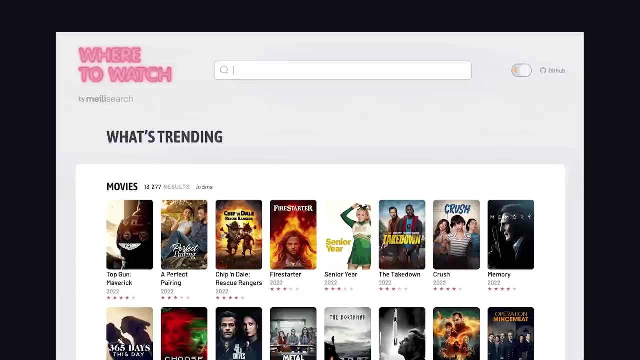 Another specialty database to look into is Meilacer. The full-text search engine space is dominated by tools like Elasticsearch and Algolia. Meilacer is an open-source, Rust-based alternative that makes it easy to implement an awesome search feature into your app. 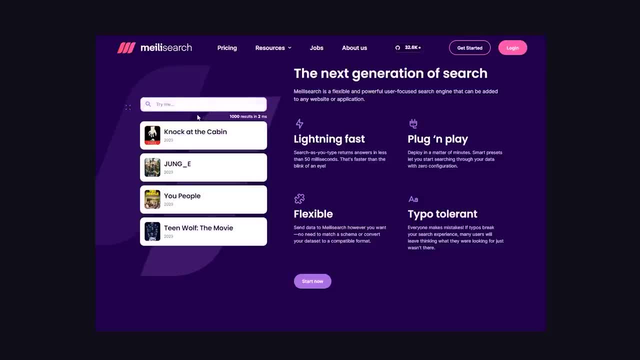 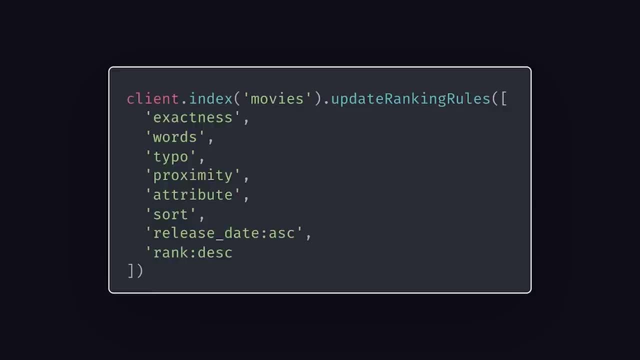 It's not a primary database, but instead a place where you would duplicate data that needs to be searchable in complex ways. like you can fine-tune different parameters to control which attributes have a higher ranking in the search. In addition, it has a bunch of client libraries like Instant Meilacer. 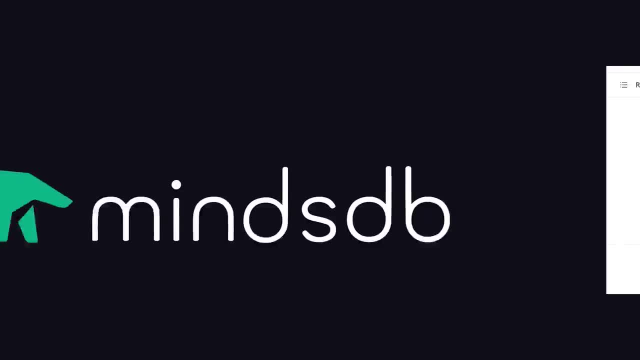 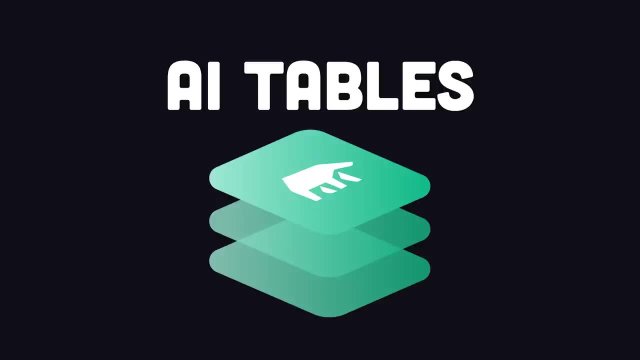 that can quickly implement a search feature in a front-end web application. And finally, that brings us to MindsDB, A database that integrates popular machine learning frameworks. It created a concept called AI tables that embed predictive models directly into the database. At first glance it feels like SQL. 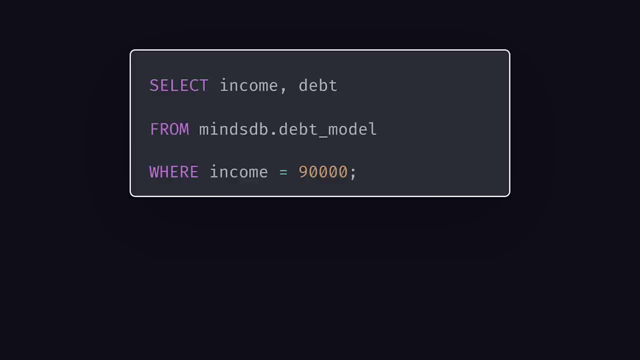 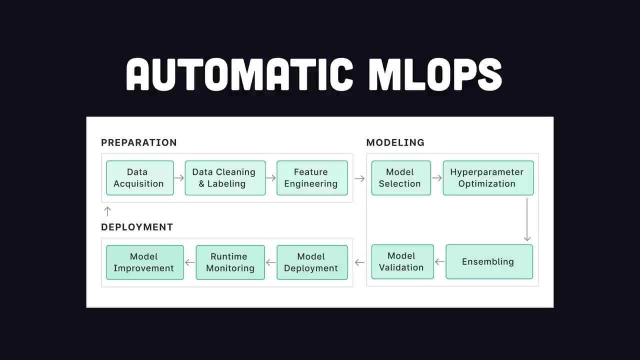 except you can use it to write statements that train machine learning models. When the model's done training, you can then use select to make predictions from it. So basically, it provides an integrated way to handle the MLOps lifecycle And it can also integrate with your existing machine learning models. 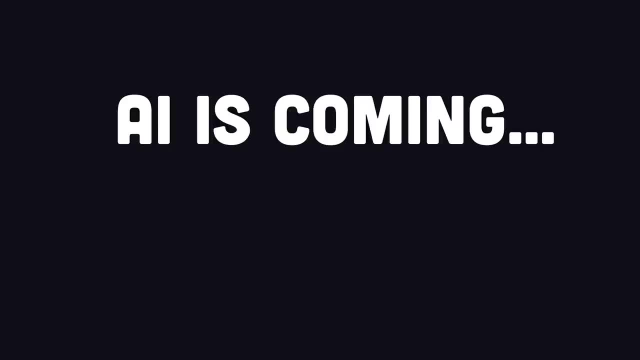 or those from third parties like Hugging Face or OpenAI. In the not-so-distant future, I believe embedding AI directly into your machine learning model, into databases, will be a huge thing, And MindsDB gives you an idea of how that could look. 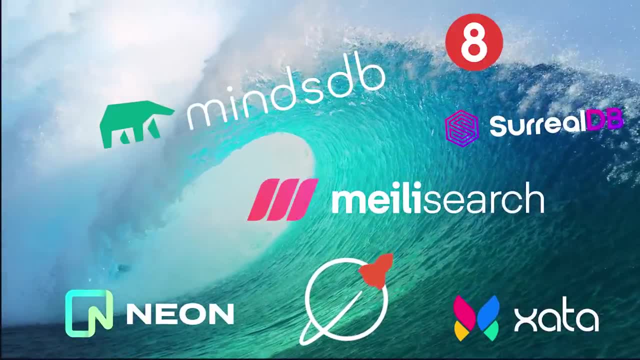 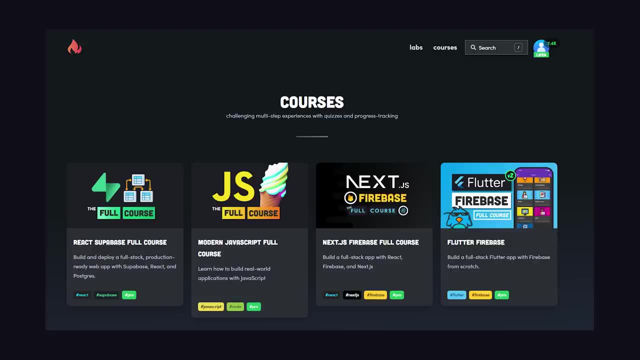 And now you have 15 different futuristic databases to choose from for your next failed side project. Good luck with that. If I missed anything, let me know in the comments, And if you want to learn more about awesome serverless databases like Firestore and Supabase, 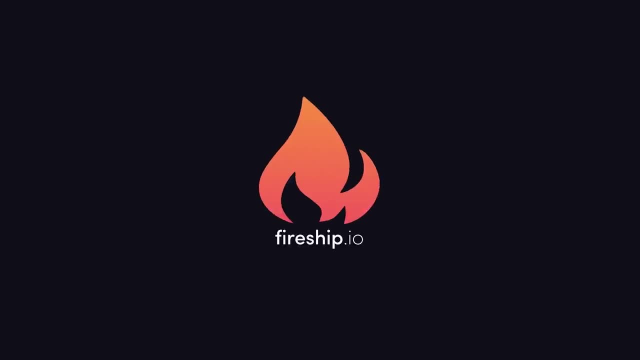 support my work as a pro member on Fireshipio. Thanks for watching and I will see you in the next one. Welcome to Math with Mr. J. 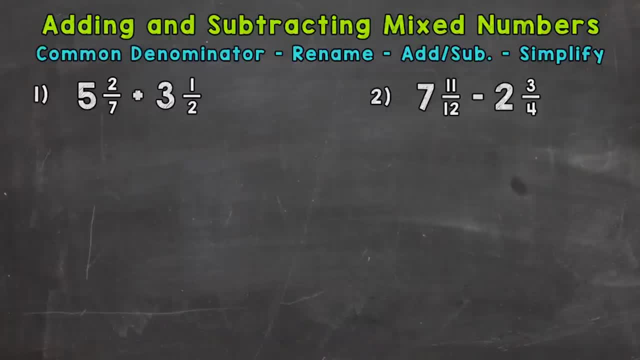 In this video, I'm going to cover how to add and subtract mixed numbers. And we have one example each that we're going to go through together in order to get this down. So let's jump into number one, where we have 5 and 2 sevenths plus 3 and a half. Now before I start, I want to mention that if you're able to add and subtract fractions with unlike denominators, you'll be able to do these types of problems. There's just a couple of extra steps, but you'll be good to go. So let's start with number one. And the first thing I like to do is line these up vertically, so up and down. 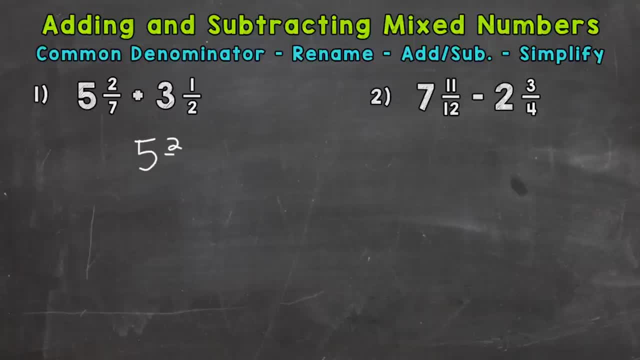 So 5 and 2 sevenths plus 3 and a half. 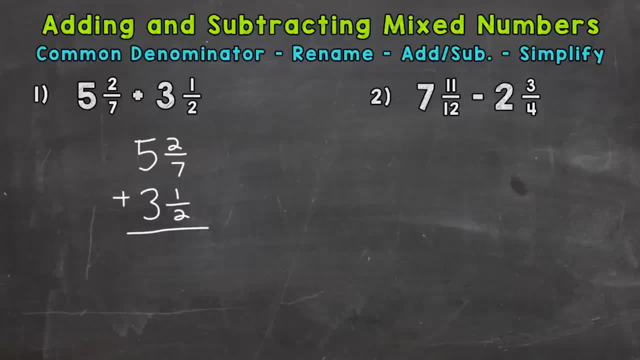 Now the first thing we want to do, we need to see, do we have a common denominator between our fractions? So can we add our fractions? Right away. No, we don't have a common denominator. So we need to find one and rename. So we have a 7 and a 2. So the least common denominator for a 7 and a 2 is going to be 14. So let's rename here. 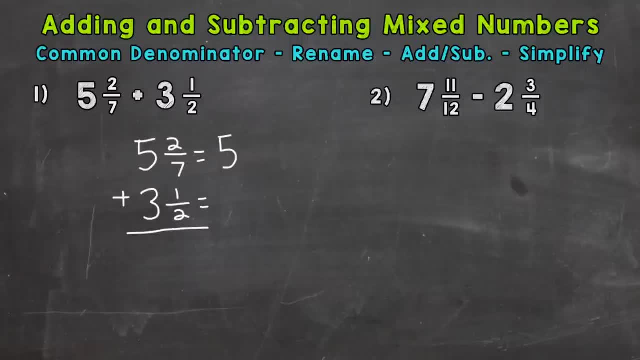 We'll put an equal sign. And we have 5 and how many fourteenths? And then 3 and how many fourteenths? Well we know 7 times 2 gives us 14. So we have a common denominator. So we need to do the same thing to the top. We're doing the same exact thing we do when we add fractions. We just have a whole number in front. So 2 times 2, do the same exact thing to the top.